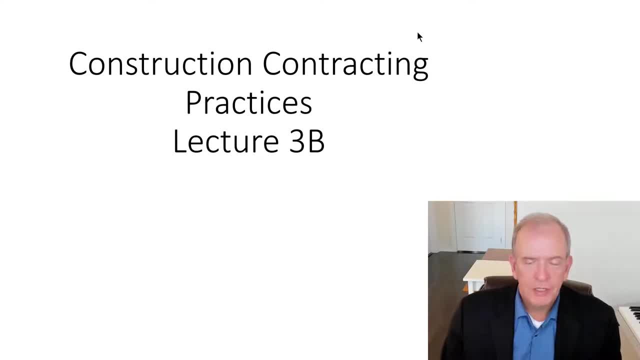 Hi, I'm Tom Stevenson and welcome to Introduction to Construction Management. Today we're going to be continuing on where we left off in Lecture 3A, So we're going to be reviewing contracting methods or procurement methods, and we're going to be looking at a 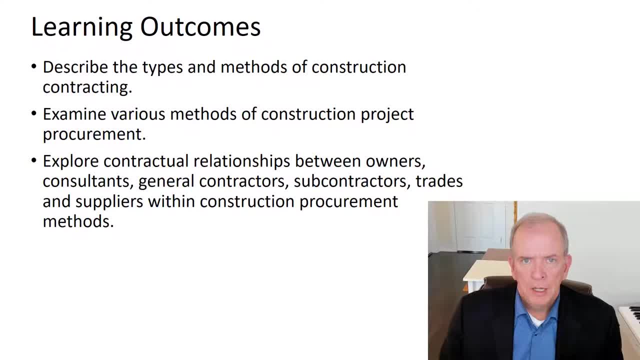 number of different procurement methods, including lump sum contracts, unit price contracts, cost plus contracts, design, build contracts and construction management, And each one of these actually forms sort of a different working relationship between the owners or clients and the parties involved, the contractors and consultants. 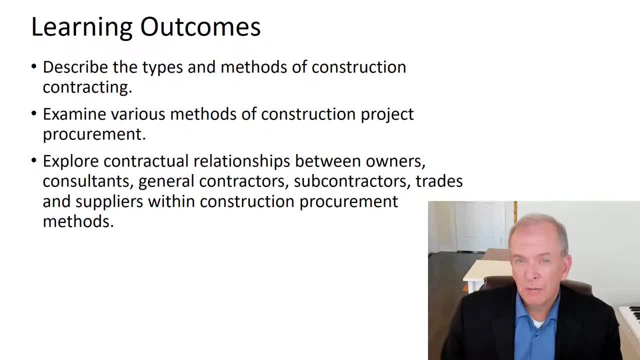 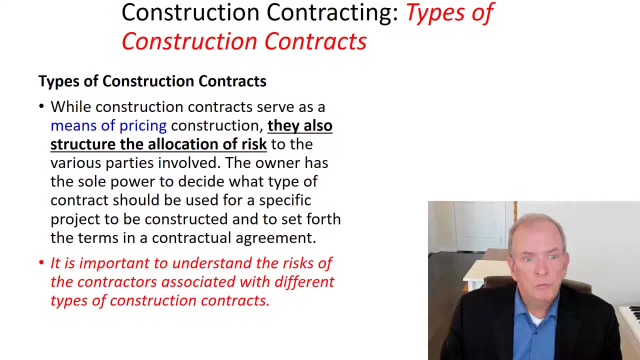 It's based on a number of areas, including the assignment of risk, complexity of the projects, how they're being funded. There's a lot of elements that come into play when deciding the contract type or the best contract type under a specific situation. So really, as I mentioned, we're trying 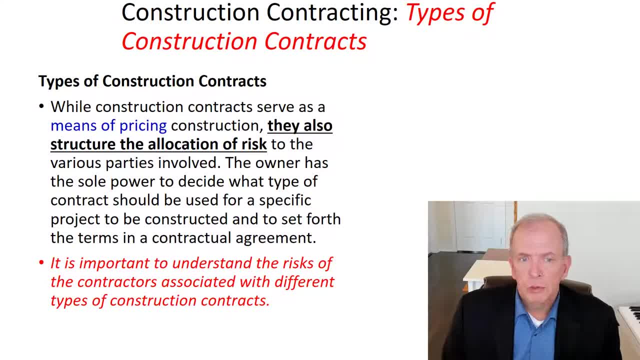 with contracts to look at how we can price the individual projects. And with pricing there's always a certain amount of risk and sometimes you know, if you take a really complex project and you want to lump some bid on it, you may find that the contractors have to pad that price because of the 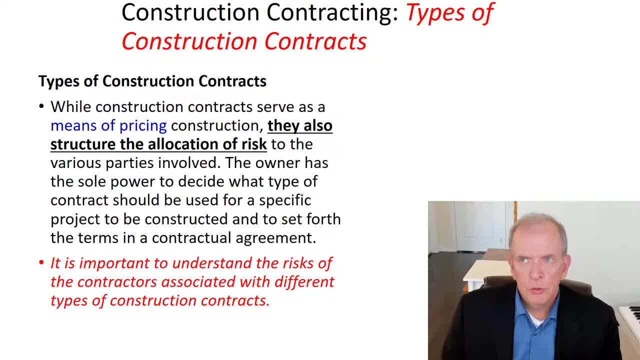 risk that they're putting on the project. So if you take a really complex project and you want to lump some bid on it, you may find that the contractors have to pad that price because of the risk that they're taking. They may feel this is too difficult or risky for us to tighten up our 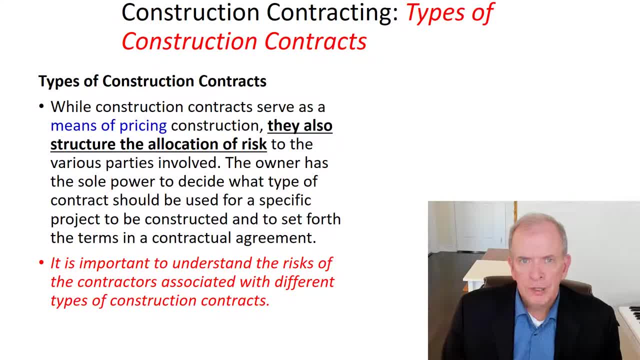 pricing and our budget on this. So what they have to do is they have to bring in probabilities, risk probabilities, do a risk log of all of the potential risks and you know what's the potential probability of this happening and, if it does happening, what's the cost of it happening. 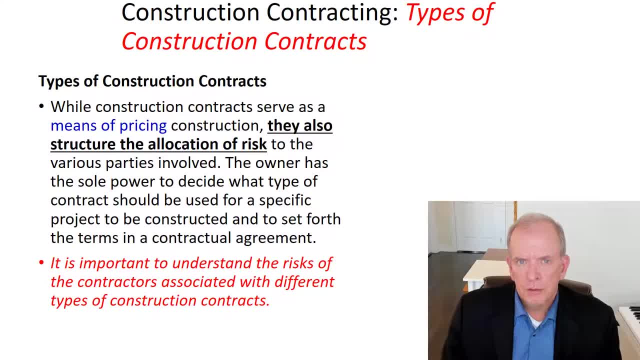 And then they have to factor that into their pricing models. So if it's a lump sum, that's that might mean that the owner, potentially, is paying a large amount of money contingent on some of these things happen. What if they never happen? Well, the contractor is going to do very, very well. 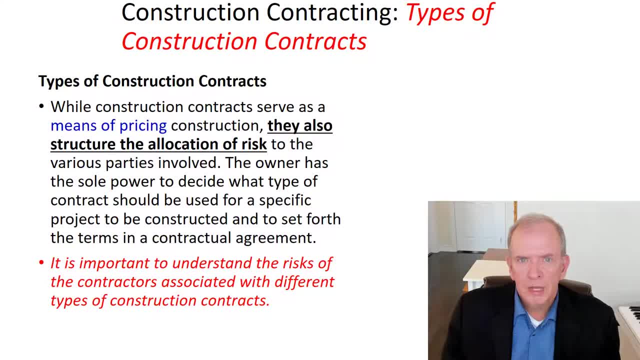 So some owners will want to not in the sense have the contractor take on that risk but pay a much higher price for it. They might want to have some form of sharing of the risk or changing the contract around, and that may potentially lower their price. There's a lot of 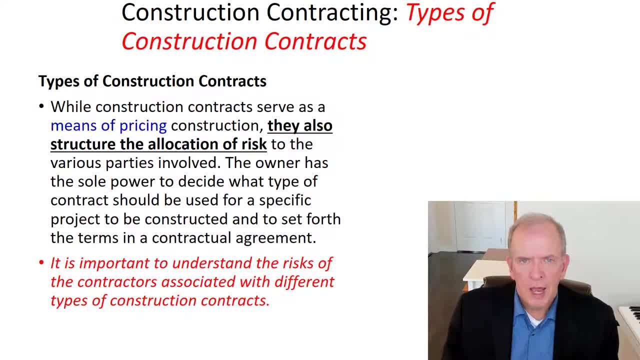 mays and ifs in this aspect, but really it is looking at the assignment of risk and responsibility. It also looks at the timing- how quick we can get the project started. That also plays into the factoring as well, So it's really important to understand the risk associated with the different 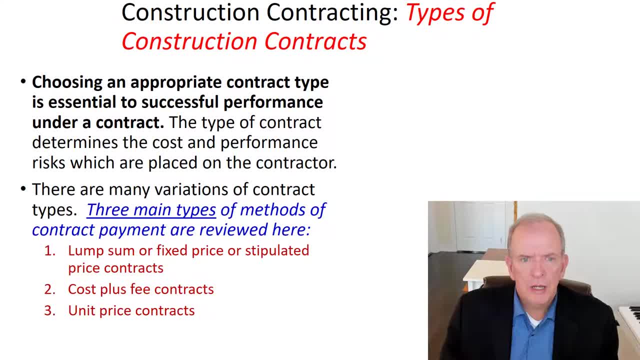 types of construction contracts And choosing an appropriate contract type is really essential to successful performance And sometimes it depends If it's a government agency. there's a lot more pressure on government agencies to use lump sum type pricing because you know you're representing the taxpayers money. 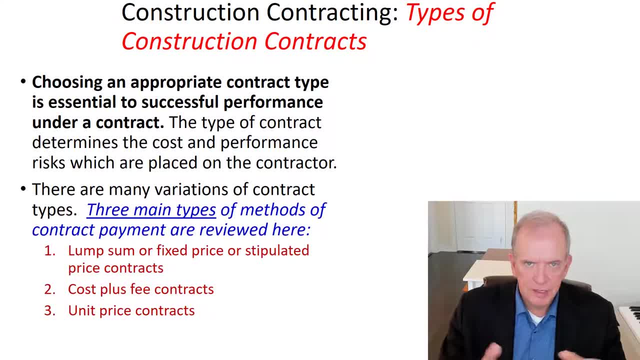 And you like to have that. everybody competitively bid on this and the process is is pretty transparent, and who was the lowest price gets the job. If they were pre-qualified for the work, everybody gets pre-qualified, But that's not always the case, as you'll see. 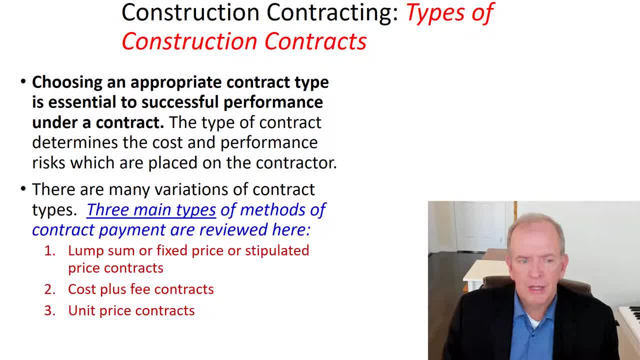 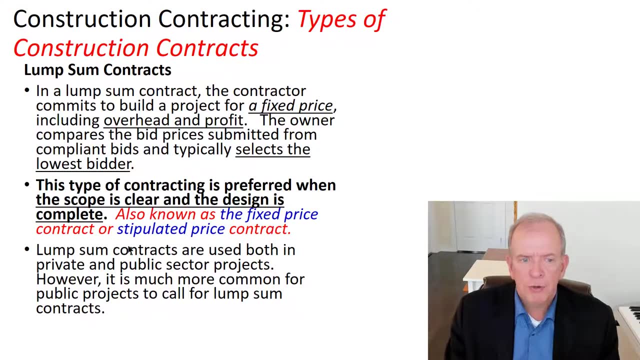 So there's the the main sort of areas that we can think about: Lump sum, cost plus and unit price contracts. Again, we'll look at some variations as well. So lump sum contracts- we've kind of already talked a little bit about that, but it can go by the name fixed price contract or stipulated price. 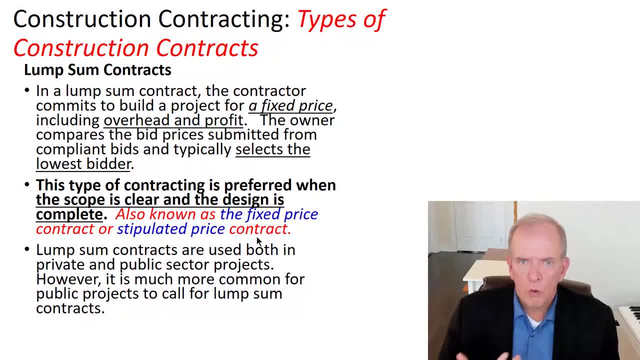 contract. It's the amount of the whole project and it's put into a price right from the get-go. So So you better have really well-developed drawings and specifications, because that's what this price is based on. If, when you get into the project, there's a lot of changes, then what was the point of going with a lump sum contract? 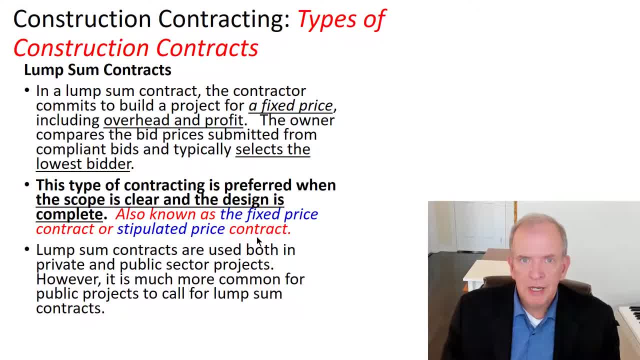 In some cases I've seen where there's as many changes and the value of the changes is 50% to 100% of the contract price. So do you really have a lump sum? in that case, I'm going to say not really, because the changes are going to have individual costs and those are going to be priced out. 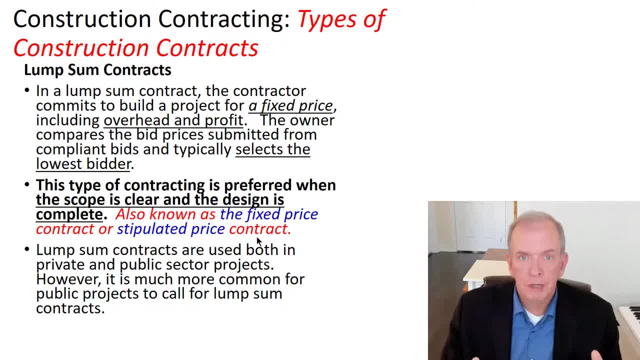 They may be priced out based on criteria that's put in the lump sum contract, But nevertheless, it's not the same as having a lump sum with a few changes. You're always going to have a few changes in it, So that's something that should be a determinant whether you go with a lump sum or some other form of contract. 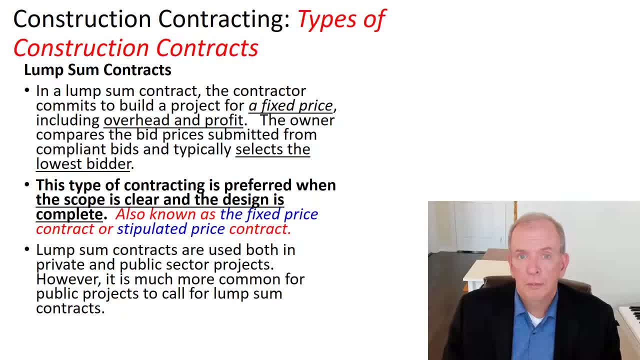 And, as I mentioned earlier, governments too. they want to protect the taxpayer And it's pretty good If they have clear drawing specifications. and here's what it is And if we can keep a tight lid on the changes, then it looks and appears, and most likely is that due diligence has been taken in the case of this building project. 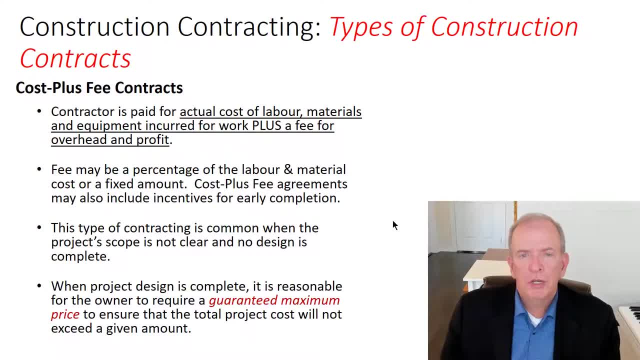 Cost plus fee contracts, So cost plus- sometimes you'll hear the term time and material and it's kind of a form of that. So really you have cost plus. So that means that your costs, which would be like how many hours of labor that you did, the material costs and then a fee for you managing that process and your overhead and profit generally as a percentage of whatever the direct costs are on the project is added to it. 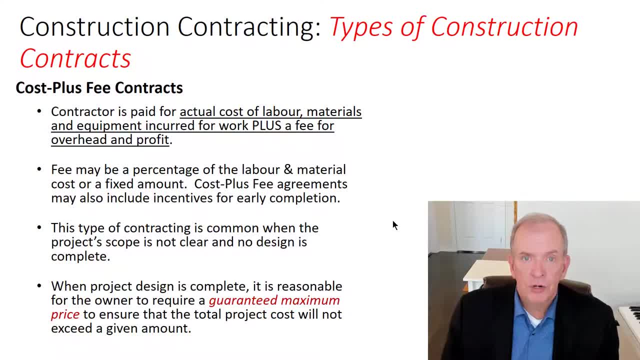 So cost plus. there's less risk for a contractor with a cost plus type contract And for the owner It means they can audit the work of the contractor. The contractor has to be able to substantiate all the costs so it can be closely monitored. 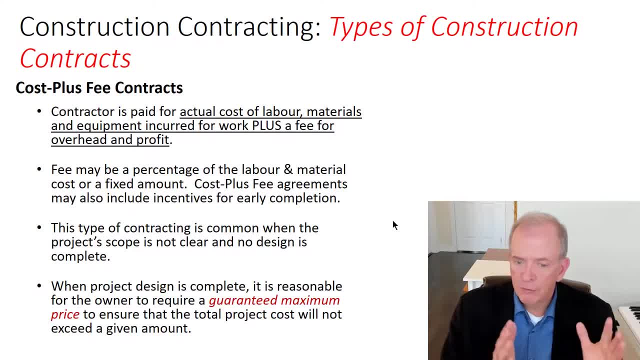 There's more monitoring goes on. If I'm the contractor too, I've got to be careful that I have everything well documented, my hours, everything well logged. that I can justify that because I always felt when I was doing cost plus type contracts- and I did quite a few of them- I always felt a certain amount of pressure to produce. 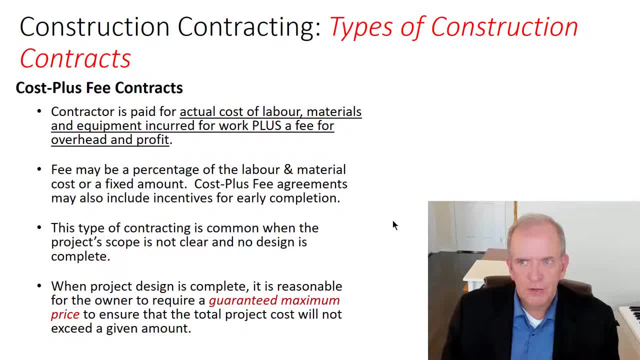 You know, clients would be Kind of more suspect if things seem to be taking longer. why are you? you know? why are you taking so long or where, whereas in a lump sum, as long as you're going to meet the milestones, they don't care if you've got 20 people taking three days to do something, even if it seems like a lot of people, that doesn't bother them. they just care that you meet their key dates. in cost plus, it can bother them because they think maybe these people aren't being as productive as they could be. 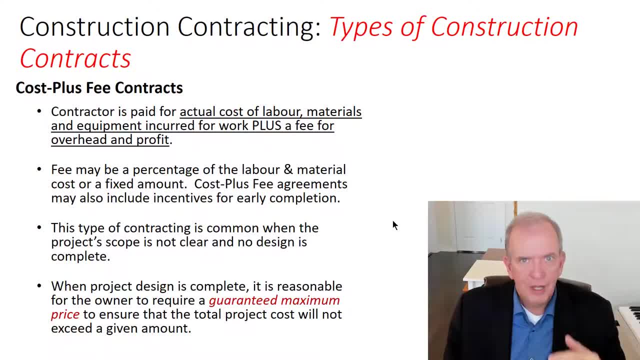 And you're, you know, expanding the overall value that you can add Your percentage, which will be a bigger percentage if it costs more. So they worry that your extrinsic rewards, your incentives, are there more to make this more expensive than less expensive. 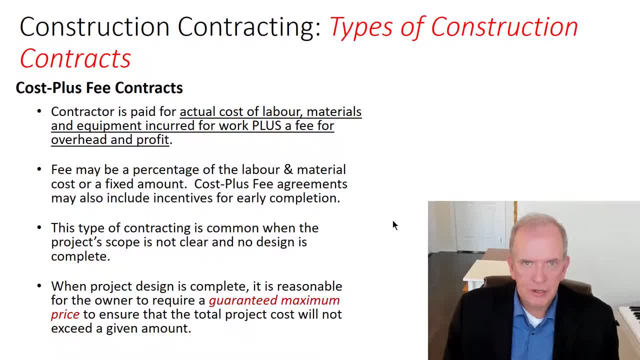 But at the same time, if you're- if you're a reputable contractor, you realize that you don't want that to happen and you want to retain this client. You don't want to have a bad relationship with this client. I always felt pressure that way. 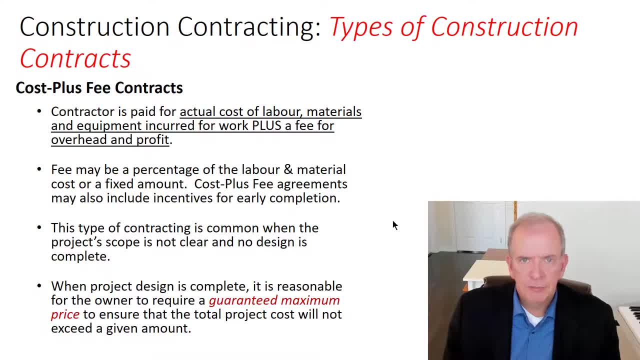 And so if we performed well, then it seemed like six months later the client had another problem. We had another project for us. Year later, the client had another project for us. So I definitely don't want to disrupt that even flow of work that I constantly get from these clients. 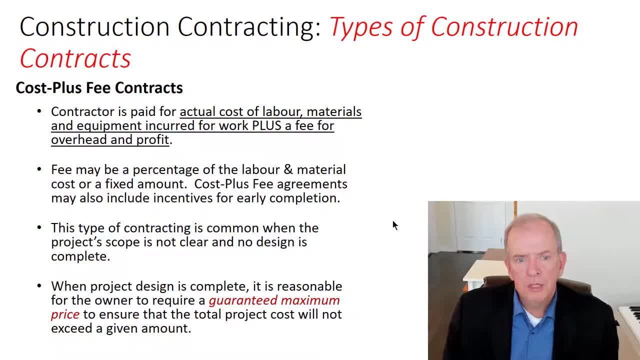 I want to be their preferred contractor, So cost plus arrangements work really well in those cases. They work really well when there's a lot of complexity and it's not this project, scope is not that clear or the design is not complete. We want to get this project done. 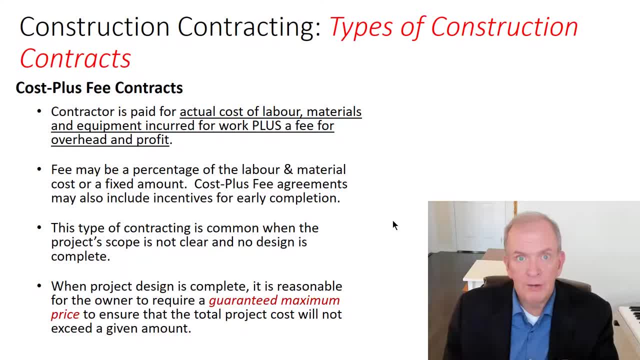 We've got the, we've got the go ahead for the foundation A permit, the substructure permit, so we can start excavating. We want you to do this on a cost plus basis. You can do that while the designs are being finished and then at a later point it can actually, if the client wants it can- fold into a related type contract, which is what we call a GMP, a guaranteed maximum price contract. 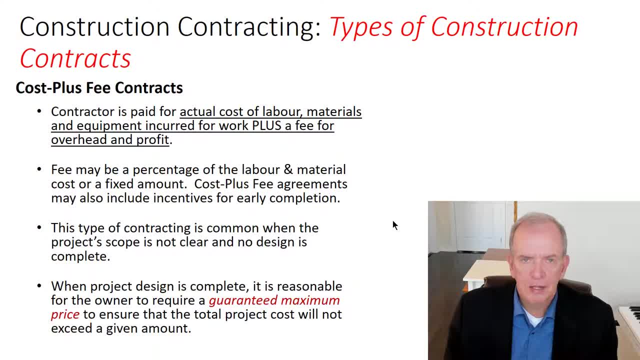 We'll talk about that later in the course- Some of these variations but guaranteed maximum price. put simply, at a certain point, when everything has become more clear, there's not as much complexity Anymore and you can clearly procure the work that's remaining. 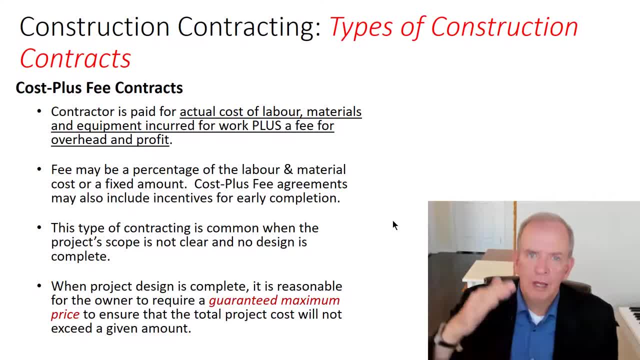 You can roll it into a guaranteed maximum price, which would mean that you have a guaranteed maximum price, that it won't go over that and you generally split the profit, That's, if you're able to do it for less than that. you split the profit between you and the client. 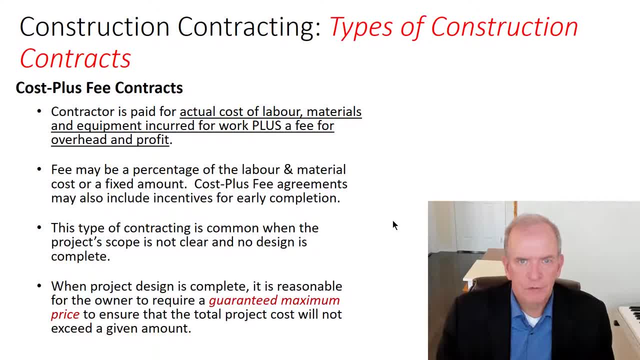 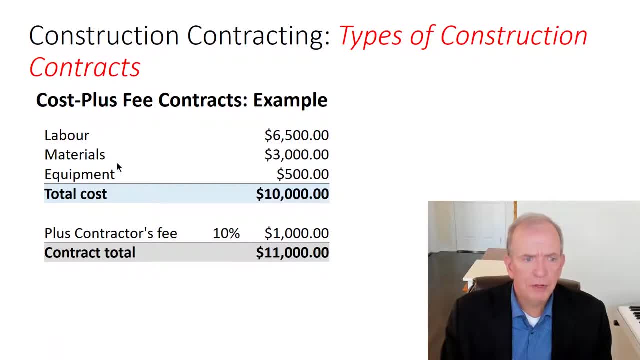 So it's another avenue that would provide some incentives for the contractor to do the work. So that's fairly frequently occurs. So you got your labor, your materials, your equipment And then you got the contract Contractors fee, whatever that number is, if it's 10 percent, 15 percent, whatever that may be. 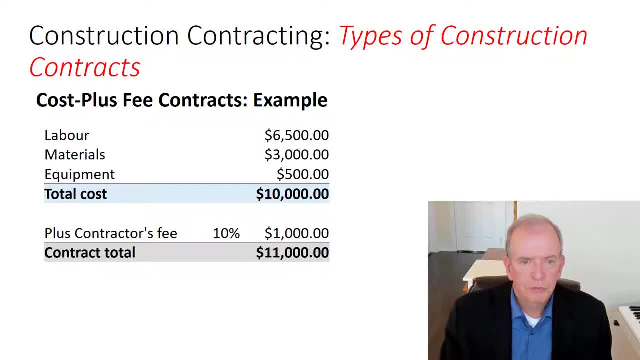 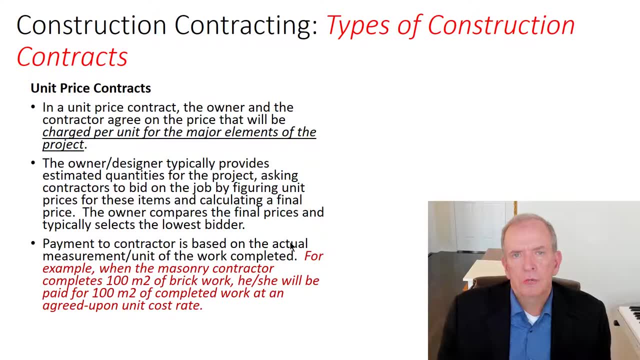 So that's just giving you sort of a breakdown example. Don't take the numbers literally, but that's just the way it works in concept Unit price contracts. This works very good. where it's something you can measure very clearly, You know how much drywall is going on per square foot. 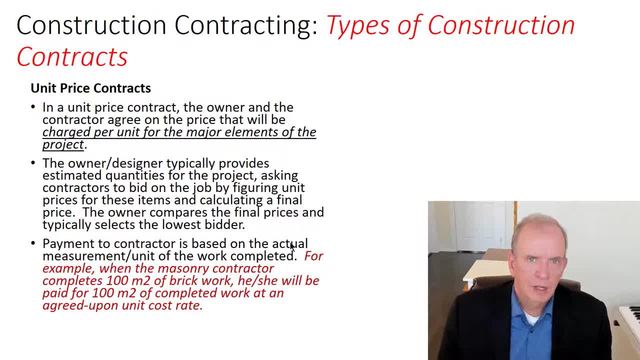 You could have a per square foot price based on how many- how many square foot you're going to put on and how how much taping you're going to do, And if it's not clear what the quantity is, it can be adjusted. So very often you might have even components in a lump sum contract, may have stipulations or contingencies in place that if you're ripping off the roof of this giant building and the subsurface needs to be replaced, it's so much per square foot to replace it. 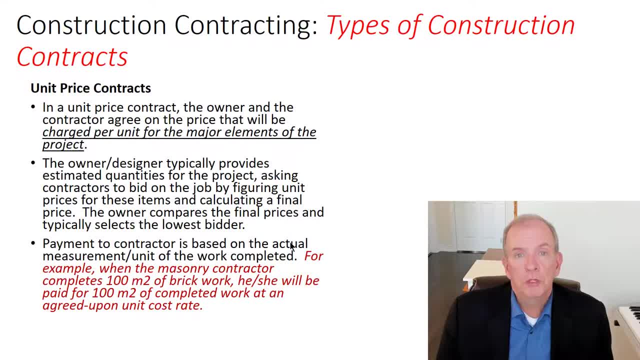